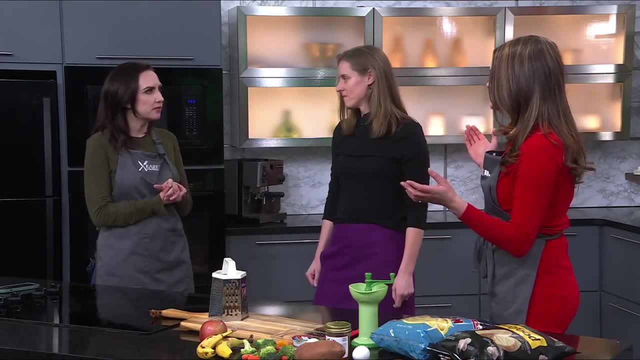 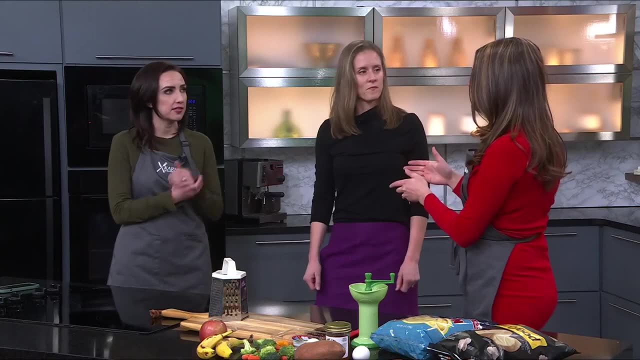 help from you. That was so, that was, that was perfect. Yeah, yeah, insightful to me. I didn't realize that they're like coughing or gagging If you can, if you can hear them- they're not actually choking- and hands off. So, yeah, I think we have to also introduce: you brought your kiddos. We already. 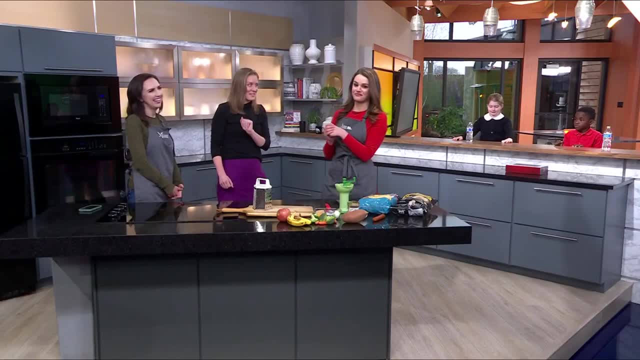 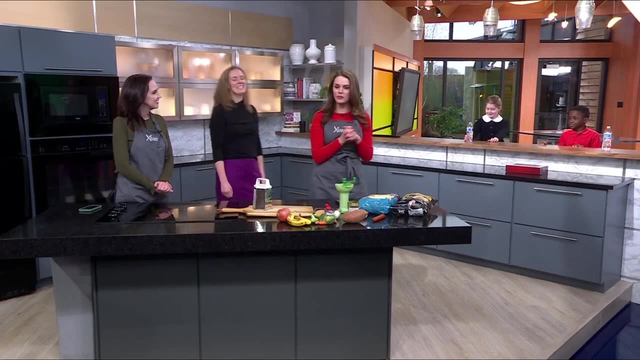 met one of them and they were a little jealous that she got to be in that one. So I've got my two back here, Sylvia and Gregory. Good morning, Hi guys. Hi, They're very well behaved because they got some snacks, too, coming their way. All right, so today is focus. 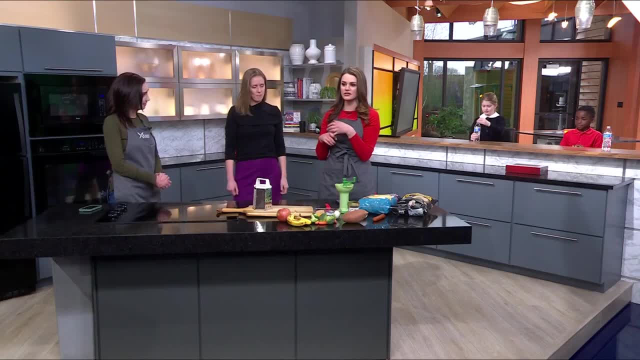 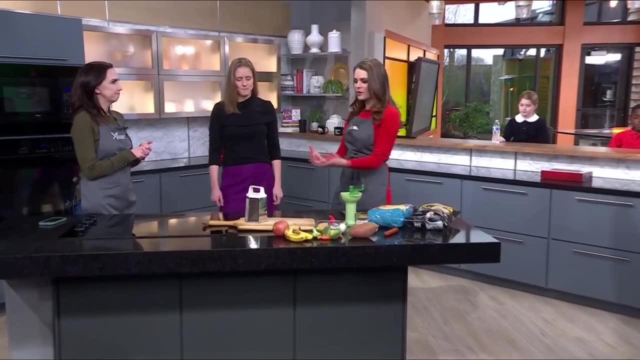 We're talking about how to chop things up, because there's certain things. babies obviously eat pureed, but they can also start eating, you know, chunks of things, and that's where I get terrified. So we have an array of do's and don'ts. I guess where do you want to begin? I would start with first, like 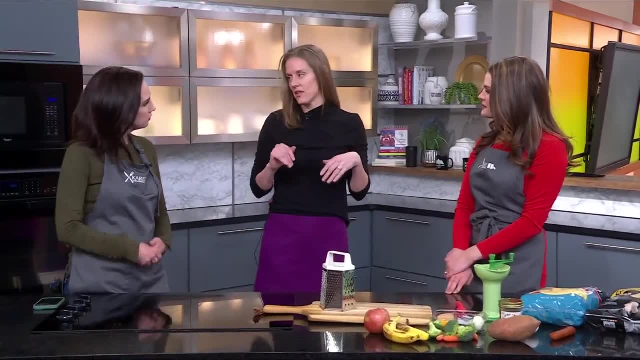 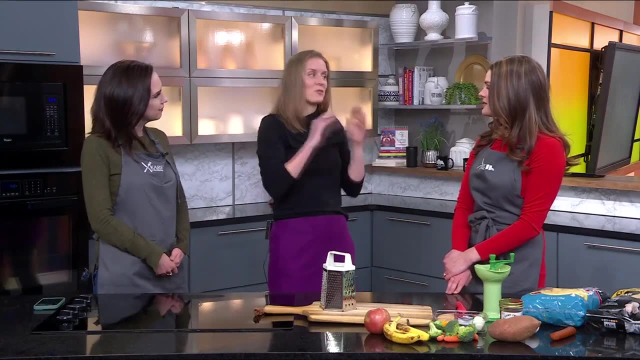 setting the tone for where you're going to eat and making sure that number one supervision and note. we're so busy we want to pop them in their chair and now is our chance to go run and do the laundry or whatever. It's not the time. it's the time to sit and be watching and be present with. 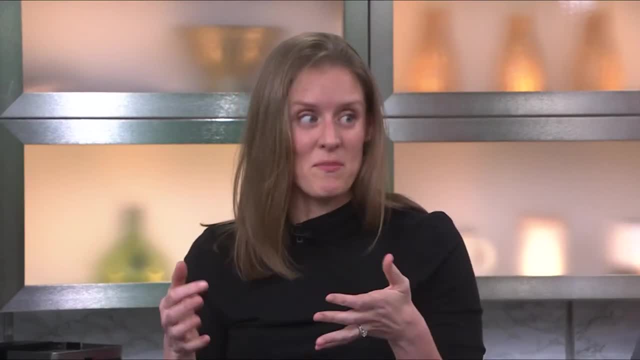 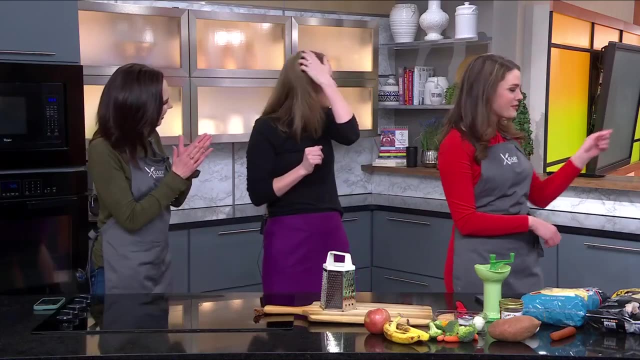 them: Supervision number one. The next thing is also like having them be sitting. We have a rule at our house that we started when they were very little and these guys can probably, if you're eating, you're sitting. That's exactly right, They remembered it. Yeah, And kids remember little sayings and they 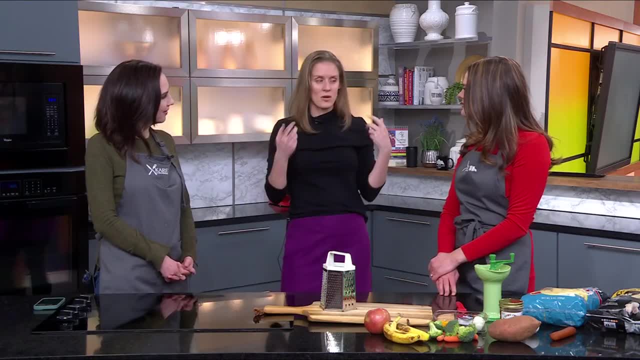 love those things. We started it really early and it's something that we always say every time we're going to grab a snack. If we're eating, we're sitting, because if you're sitting you're not running around, You can't inhale something. That's smart: If you're eating, you're sitting. 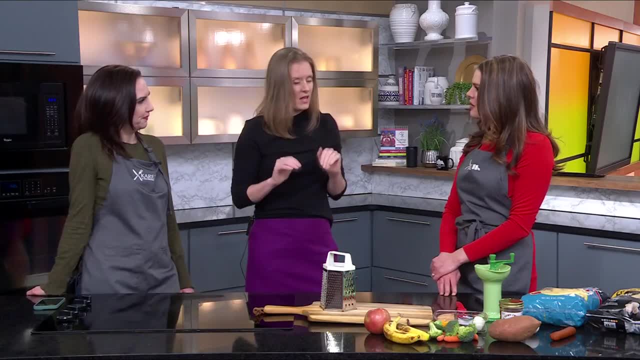 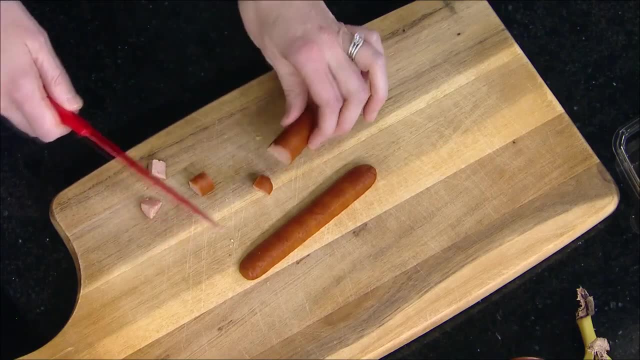 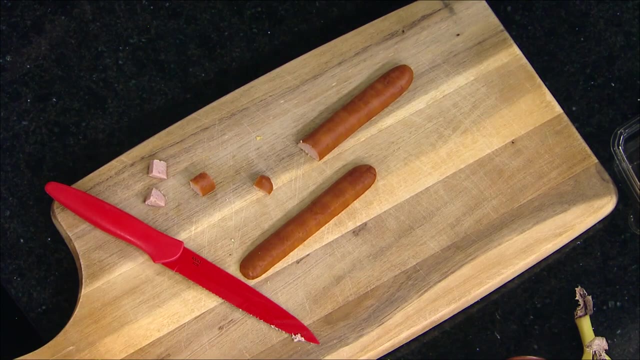 Okay, Sitting and supervised. So that's the start. Okay, Then the big things about it. You just it's such a small, much more smaller, manageable piece. If you cut it in a circle, that's the perfect shape to get lodged in your airway. So, as long as there's some ways air can get through, 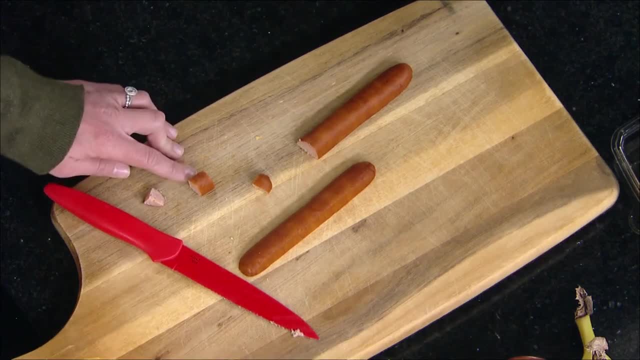 and get around it. I mean, I feel like these are even- I'm like still terrified of even this, I know. So this is good. Smaller than that even So, that's okay to give to like a six month old. I wouldn't. 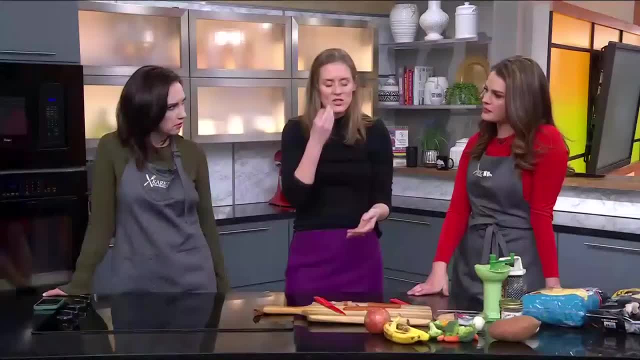 do a six month old probably at this age I'd wait until you're closer to a year where they can really like. It's just all about the development of that kind of chewing tongue motion, And that takes a while, And really not until you're about five or six months old. Yeah, And then you're like: okay, I'm going to. 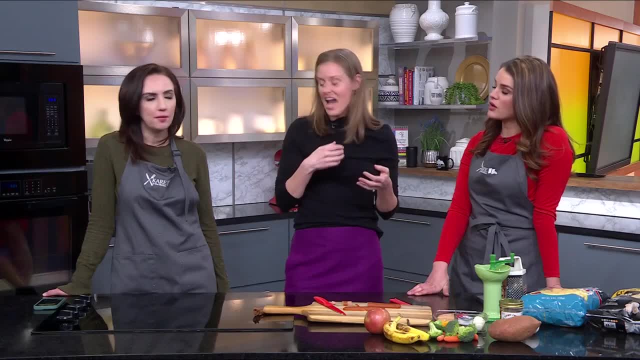 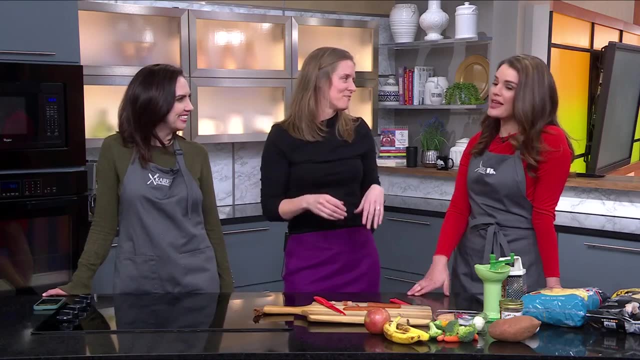 wait until you're about four, as when you're really good at all. Wow, I know. So we're cutting these things up until they're four. Okay, And I know that sounds old, But I mean at that point, You're used to it, They'll be used to it. You're used to it, They're used to it. You're just cutting things. 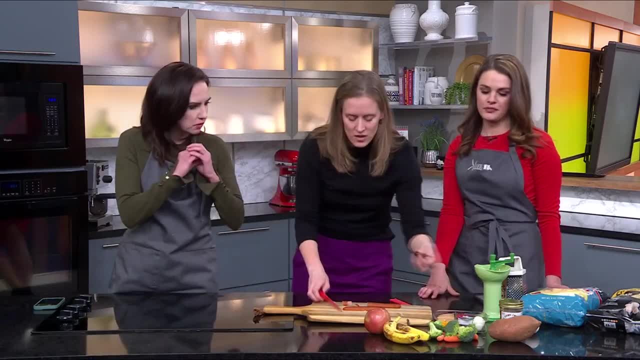 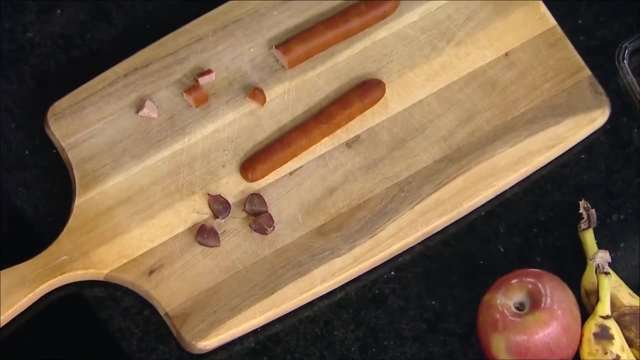 up till they're four. Okay, Is it the same rule for like grapes? You're just trying to avoid that. You're trying to avoid that shape. Yep, So definitely lengthwise for sure, But then again I would quarter quarter it. So quartering things is a good option. I've also read online And this: 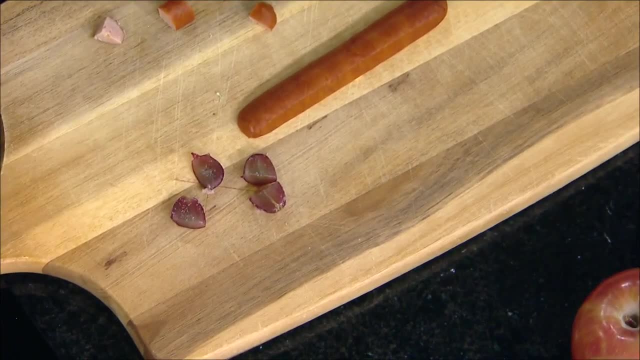 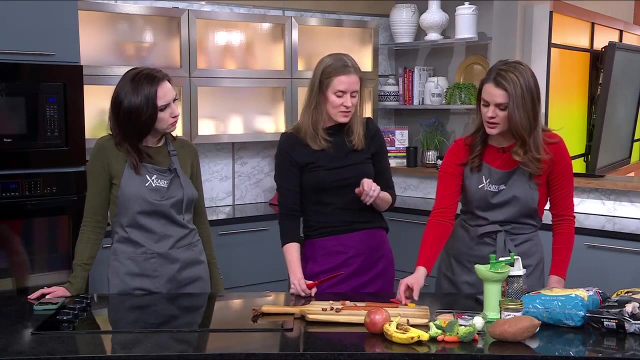 is even for infants. I was. it was like they can't cut it. I think they can cut it, I think they can. can start having soft cheeses and like cube cheeses and I think I'm just like. I don't think my kid, my eight month old, can chew this yet. so what about cheese? a big chunk of something like: 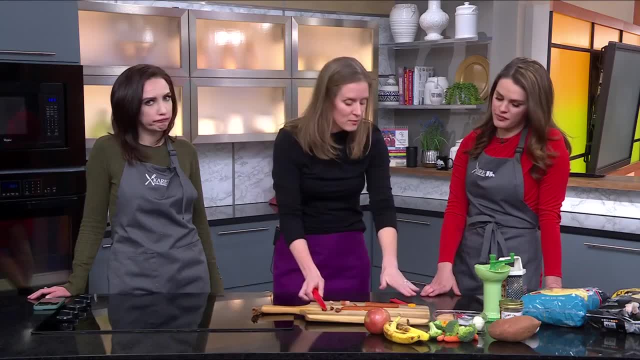 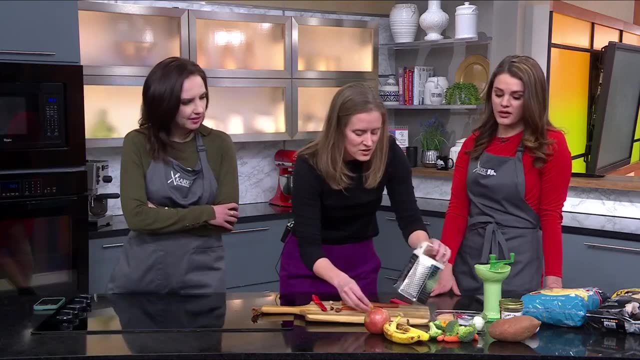 that when they're really little, that's going to be hard, it's going to be hard for them. I recommend shredded cheeses or even just taking a grater and, with your chunk, just give it a good shred, because these, these are little manageable pieces so baby could eat that. wow, okay, yeah, same thing. 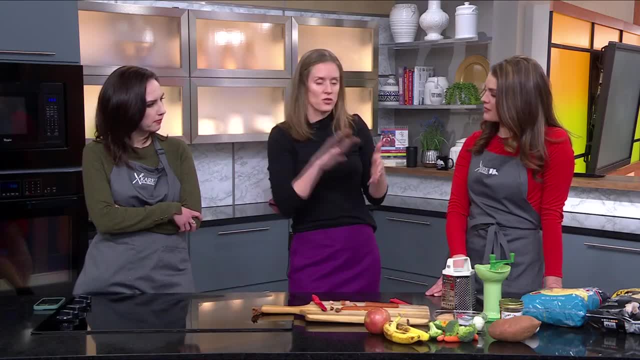 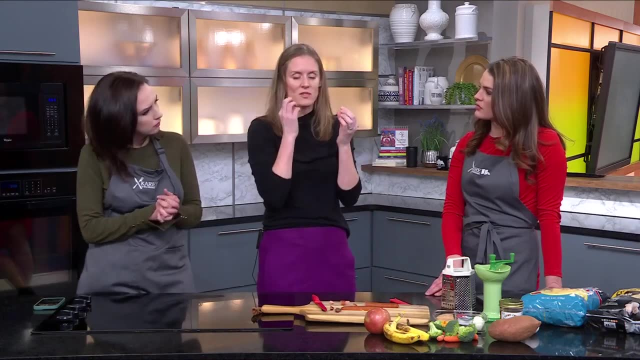 with, like your, your fruits and veggies. those are gonna be really hard until you get to that kind of 14- 16 month range, and even after. then you're gonna want them to be like a soft, squishy consistency, because they have to be able to squish it with your gums, essentially so like a rock here. 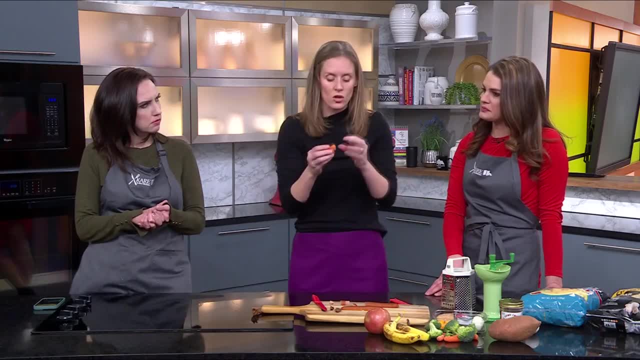 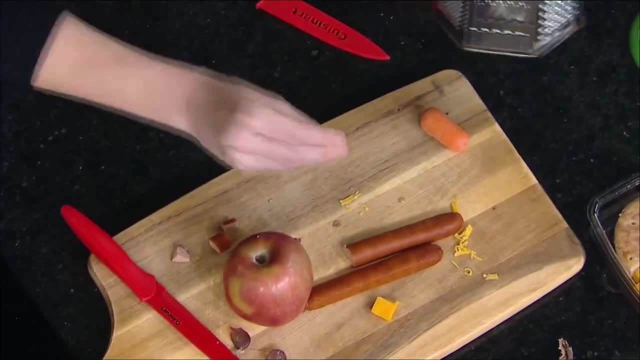 we're never gonna give a raw carrot to a little one. okay, you could cook it like cook it down a little bit and shred again with your grater tiny chunks that they can grab, can you even give? so what's the age range for the shredded apple? the shredded apple again, I would. I don't. 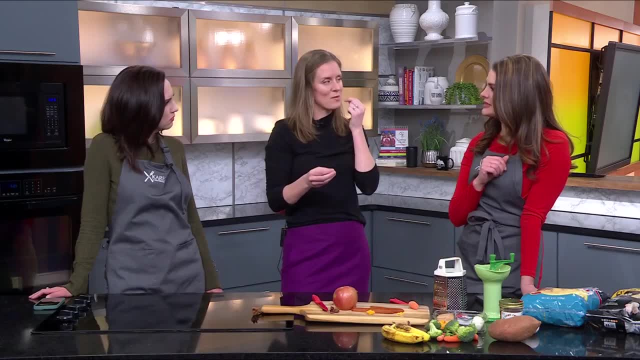 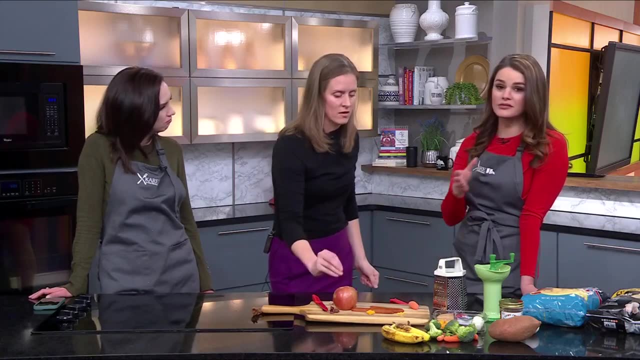 know, and it's all going to depend baby to baby. but if you feel like they can get it in there- kind of gum it a little bit, then you're right. and again, anything you feed them- if you're watching them right, you're right and I feel like sometimes they. this is where I freak out and I start hitting. 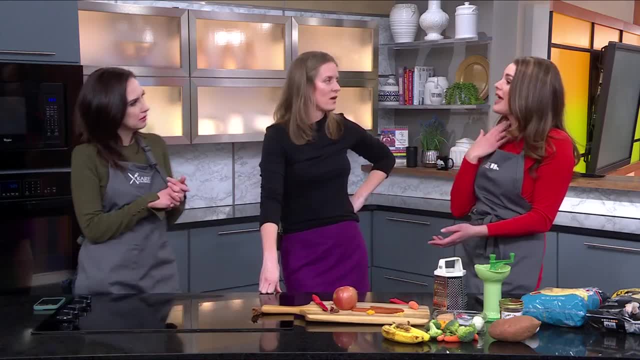 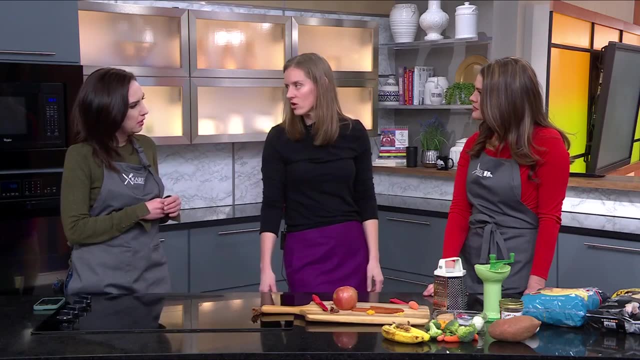 my kids in the back when they- because I could see a shred of apple- maybe the gig right and they're they're meant to gag. their gag reflexes are great. they're. they're designed to do just that: to gag sputter and to leave your hands off them when they're doing that is so counterintuitive. 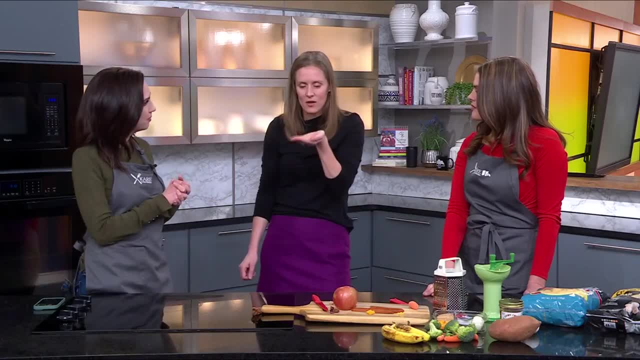 to what you want to do it as a parent? yep, you want to touch them, you want to do something. you want to touch them. you want to do something. you want to touch them, you want to do something. so, putting that hand out in front of their mouth is a good way to help, because you, it's something. 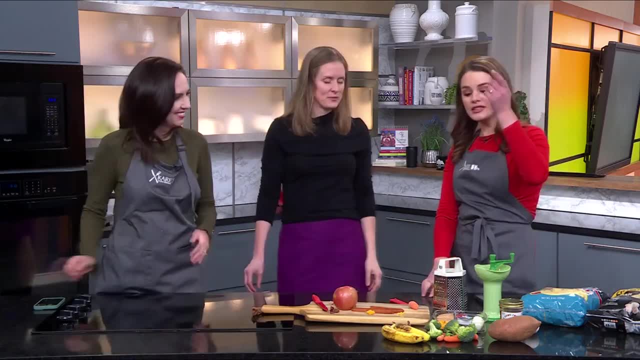 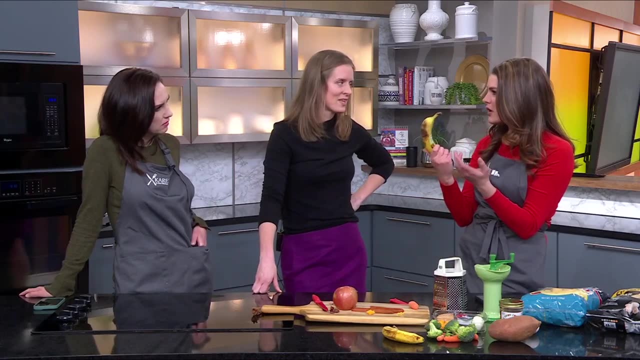 you can do here, go ahead. yeah, another thing I saw, so I saw mine, like you can give, you give a banana and you can like peel it a little bit and leave it full, but that terrifies me. so how do you, what would you recommend? it's again your comfort level and how good do you think your baby is with? 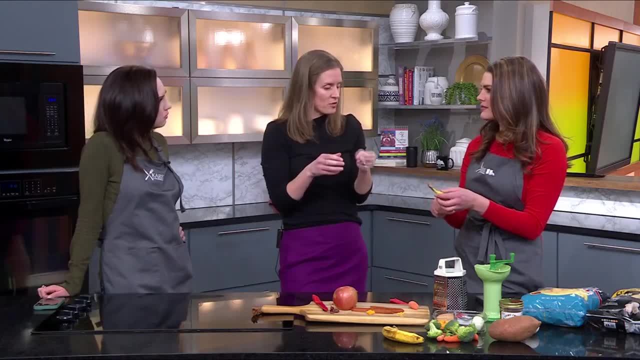 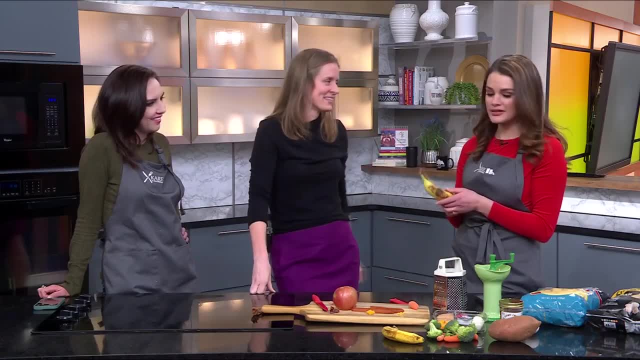 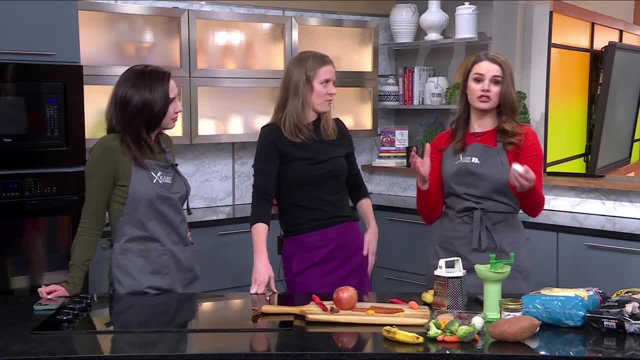 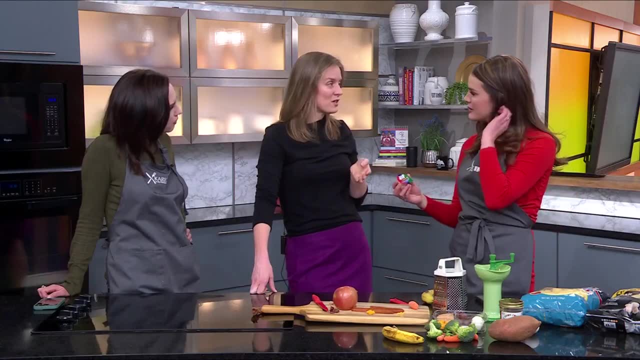 peanut butter. this is a big one, new parent even, because allergies, um, i feel like parents this, and it's different from pediatrician to pediatrician what you hear. so what do you recommend? yep, you want to start getting those allergens in pretty early because there's so many of them, and you 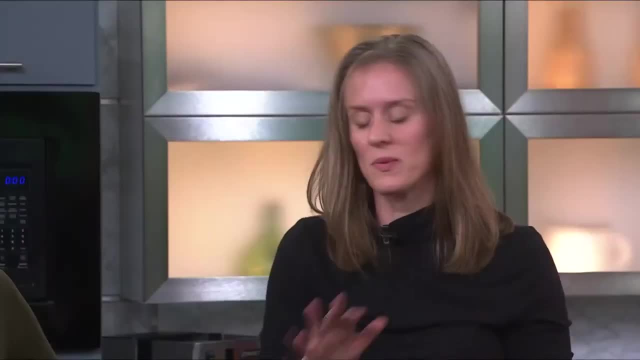 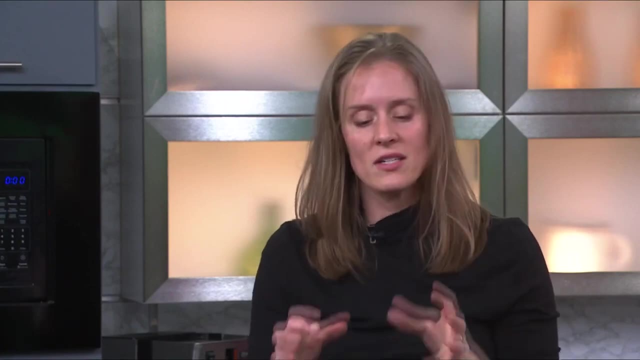 need to kind of do one and wait for a little bit before you do the next one. so peanut butter is great. spreading it very, very thinly or mixing it in with, like their oatmeal or their rice cereal. um, chunks of peanut butter, big scoops, big spoonfuls of peanut butter are a no-go, because 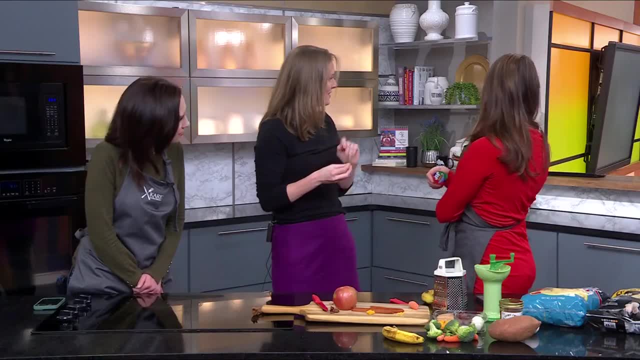 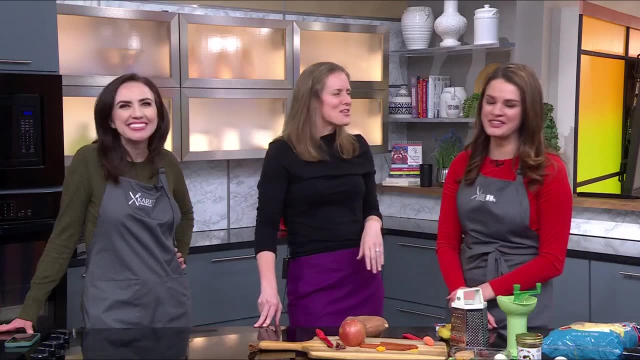 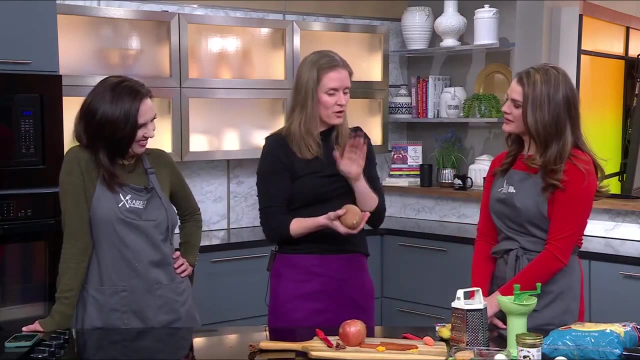 it's so thick and chewy. do you guys like peanut butter? yeah, yes, it's safe. but that's what i did. i blended it. i know, yes, okay, so we're not alone. even doctors do it. no, they're just like us, exactly. so this, you're gonna stick it in your instant pot, you're gonna bake it, whatever you. 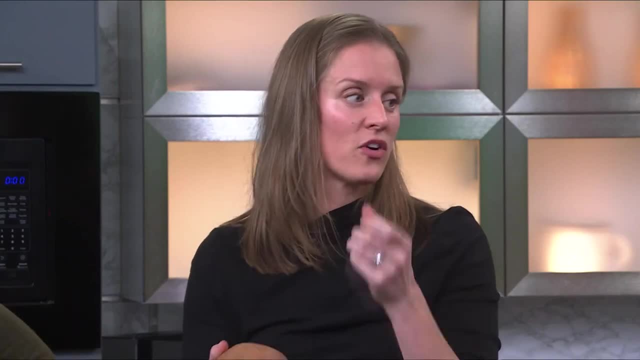 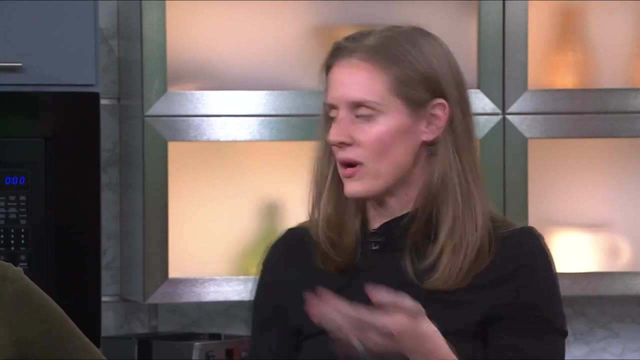 do with your potatoes, and then you're gonna again squish test. so if you're gonna give them a big, big chunk of it, like a long strip of it, thin and squishable, and if they can squish it, then you're gonna be okay, they can grab. 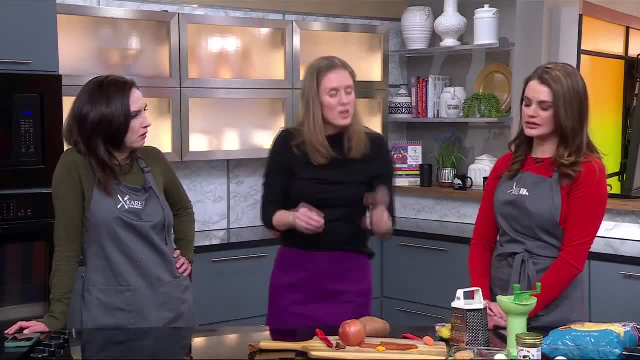 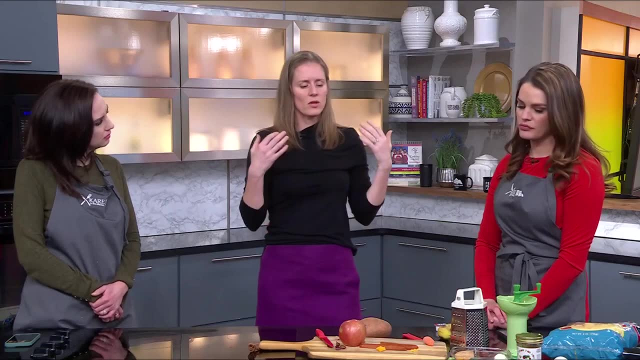 it and bite it like a fry. essentially, yes, exactly. but you don't want it to be crispy like a fry, so it's got to be squish, squishable. and then again with little ones, especially with the baby lid. we need people, you know, want to feed what they're eating, that that can introduce a lot of like salt. 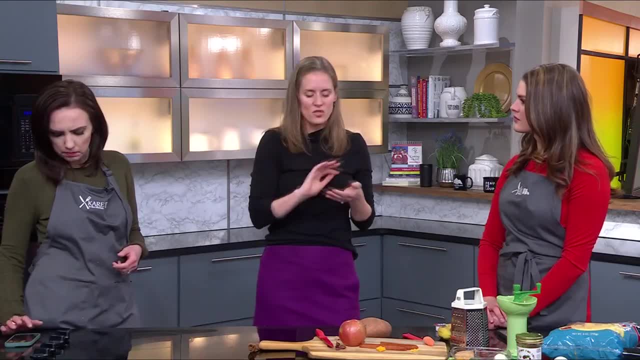 and things like that. so unseasoned, but it's a seasoning sign, but not a lot of salts, not a lot of added sugar. okay, any questions coming in on facebook? not quite yet, but i had a question about popcorn because i feel like that's the number one thing that's going to be on your list of. 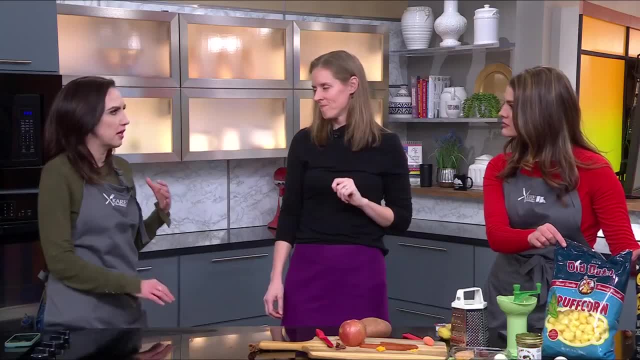 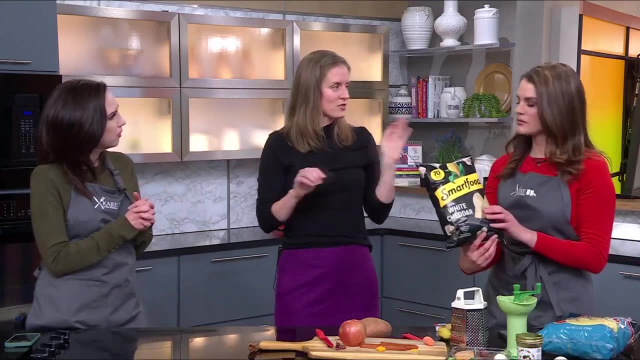 things that you're told. i remember our pediatrician when we had our first saying like no popcorn till they're five. i'm like: are you kidding what? what is the big deal about popcorn? hot dogs, grapes, popcorn- those are the big three. um, popcorn, it's got the kernels in it, it's just the nice perfect. 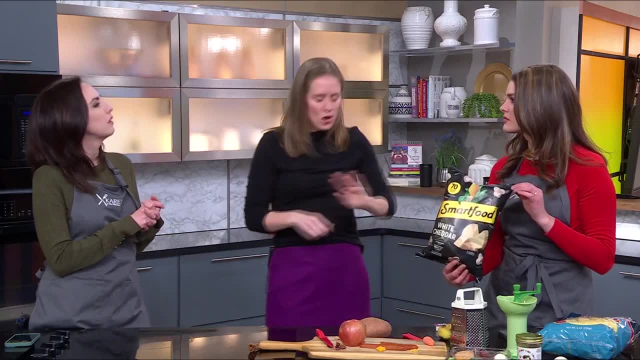 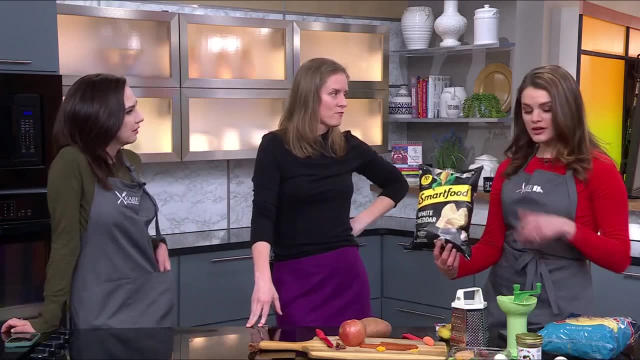 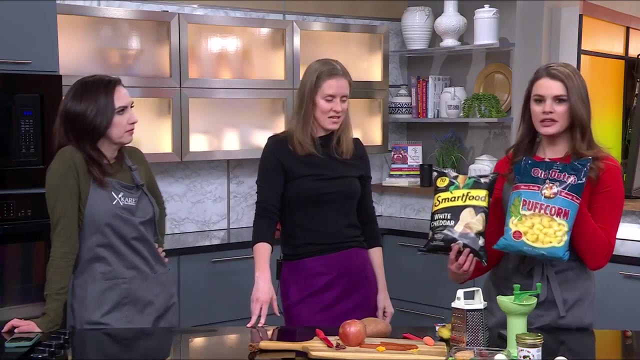 size, it's light, it's airy easy to do one of those with it. no popcorn, um until when? until four years? yeah, that's the american academy of pediatrics recommendation. so as an alternative, would i see this online popcorn. popcorn, it like dissolves, it, kind of melts in your mouth. okay, it's like a teether, a tether strip. it's. 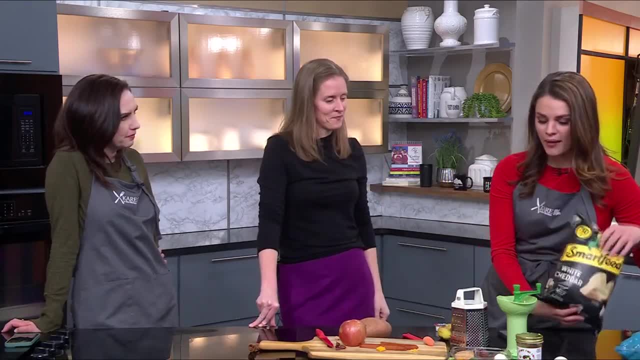 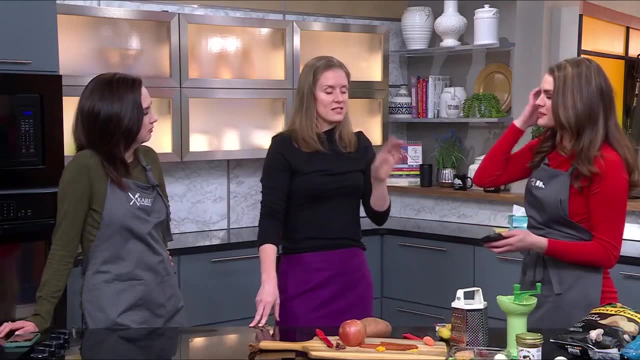 exactly like that. all right, so the no's and don'ts of that. um, i do have some questions from. we got so many people on instagram that had questions. can i just say one more thing about popcorn? oh yes, please, this is, this is a really important one, because this is what we actually see quite often, is they? 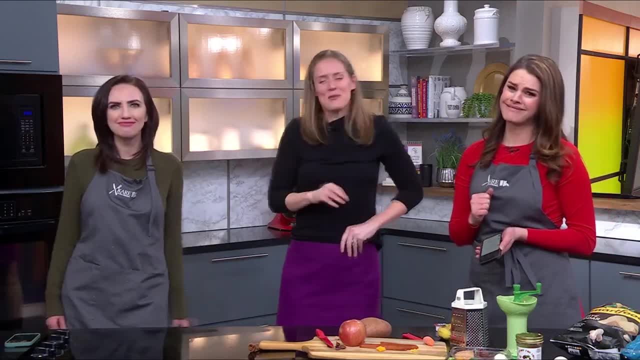 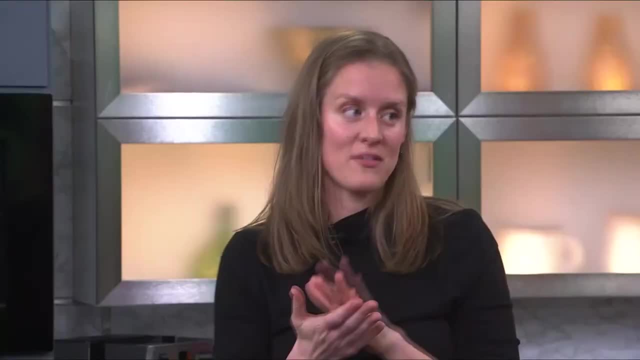 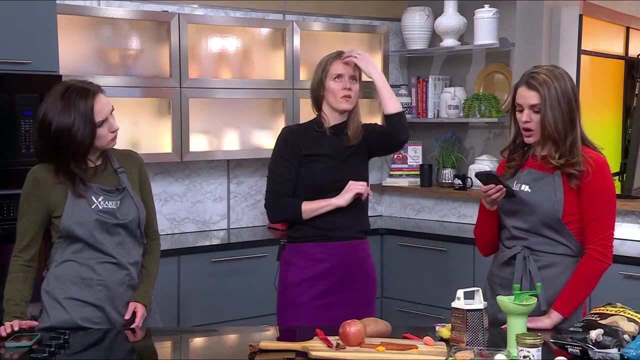 went to the movies with grandma, grandpa. oh so, grandma, grandpa, they love you so much and they want to give you whatever you want, and so make sure you're talking to the others in your family. popcorn is a no-go. popcorn is no evil like it would be that, for example, small piece of avocado. 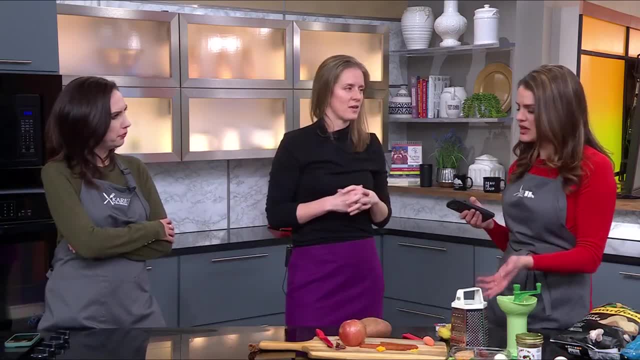 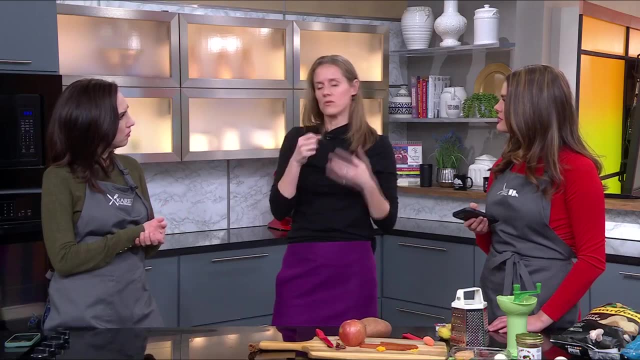 or do we give them the entire slice? kind of the same idea with, like, i guess, pretty much anything. yeah, yeah, avocado is one of those that passes the squish test nicely. so if you wanted to them to hold on to it and you're you're committed to doing the baby lead weaning thing, that's fine. so if you're 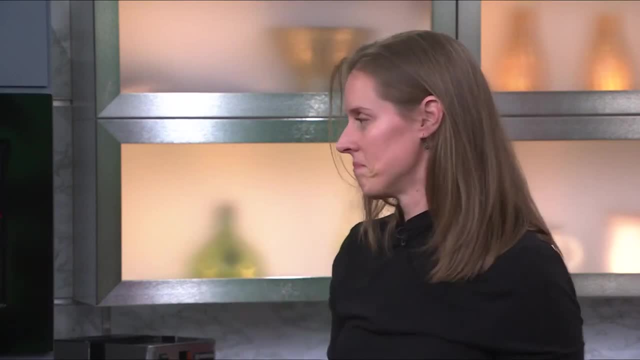 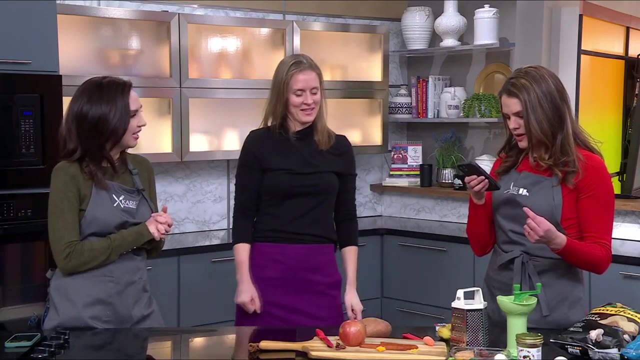 right there watching they can pass the squish test. you're okay, squish test, it's very important. i got to start squishing things more. um, lots of squishy. what else do we have? i actually had one that i thought i had never thought about this. so if your 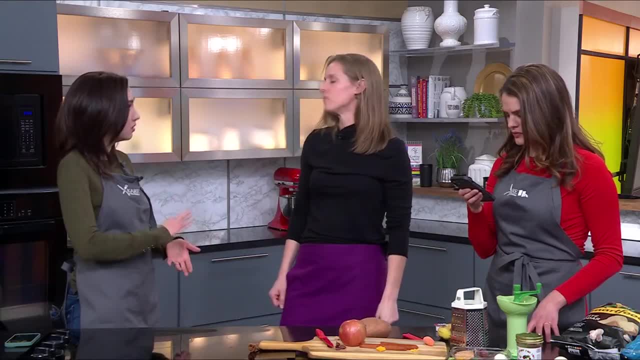 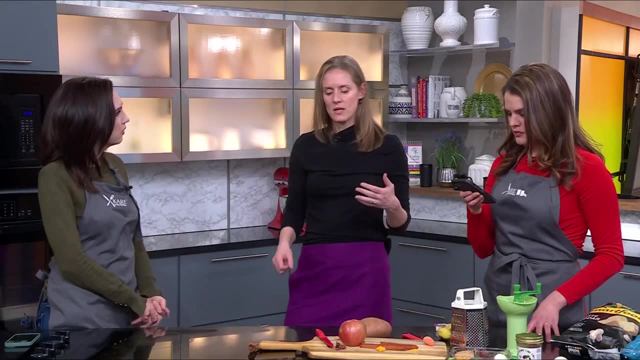 child does truly choke, and you successfully, hopefully. you know you are able to get that out. do they have residual damage from the choking? no, no, the things you're going to watch for would be like, if you're worried that some of it still made its way down, then you're worried about it coming. 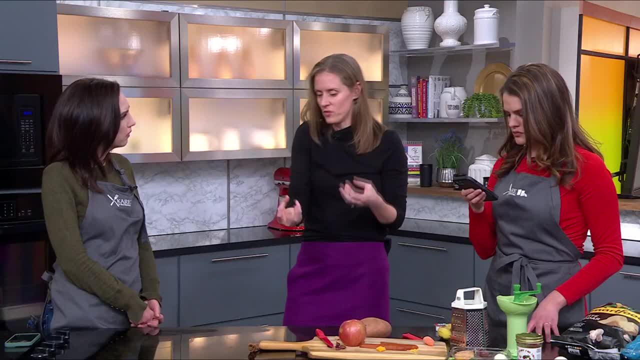 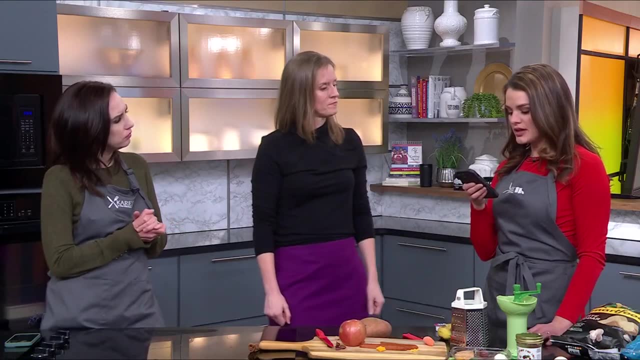 up in the future, some like a pneumonia or something like that, but most of the time, if the food came out, you're fine. okay, there's no like scarring to their throat, okay, steph had a question. she said it's a debate in her house between her and her husband. at what age can we stop cutting? 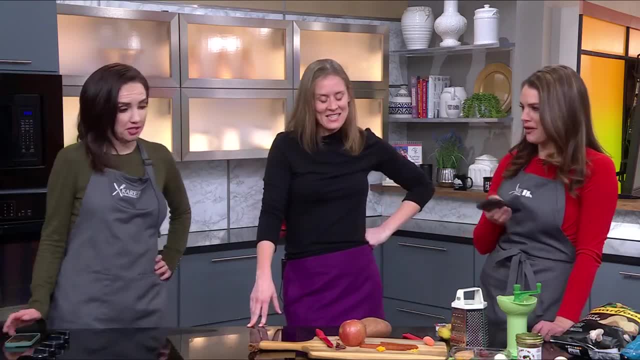 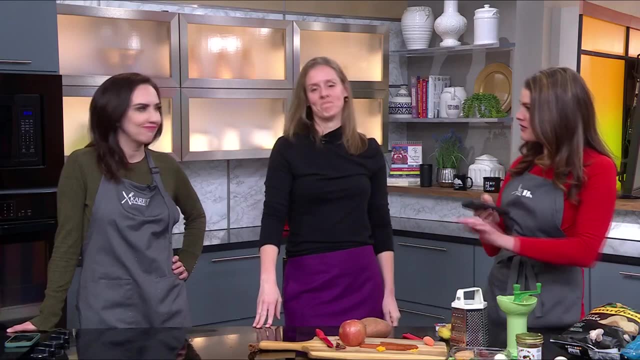 up grapes silly question, but i want to settle this once and for all. not a silly question and the the true answer that if you're going to do a multiple choice test, it's going to be four years old. four years is kind of the. that's it. that's like a graduation to you figured it out, that's. 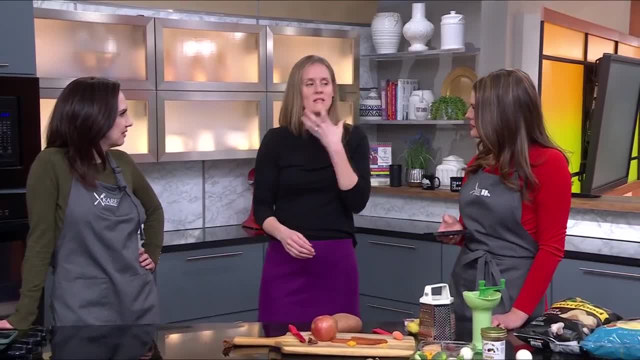 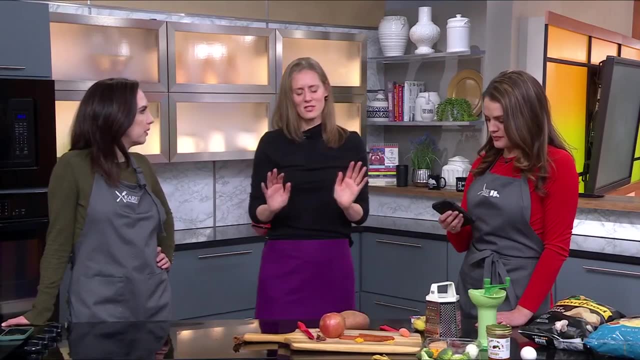 when those oral motor skills, that development is in place. and for most kids again, it's like you know your kid if you, if they're still sputtering and gagging every time you give him something. but just just wait, there's no hurry, just keep cutting it up with easter too, right around the 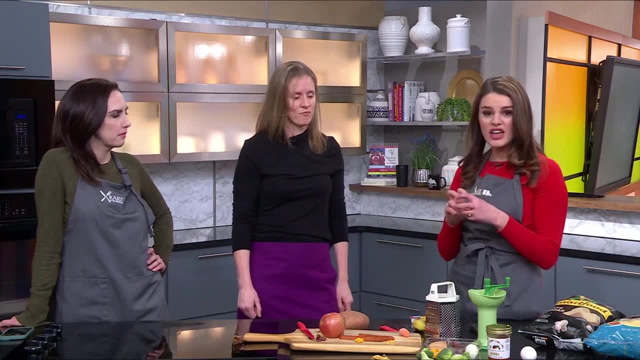 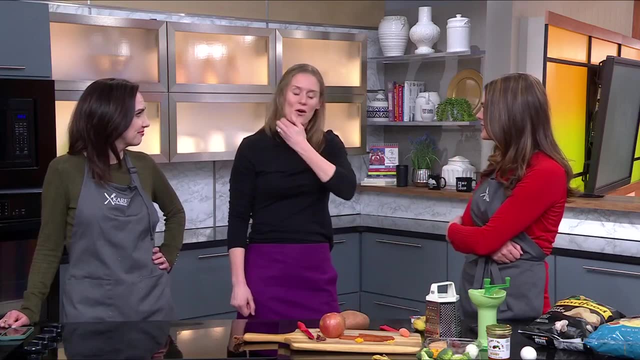 corner there's all those little like cadbury eggs, these candies, these hard candies. i feel like with parents and like jelly bellies and jelly beans. yep, what is the rule there? hard sticky candies are a no-go, a jelly belly you'd really have to kind of really hard to squish. 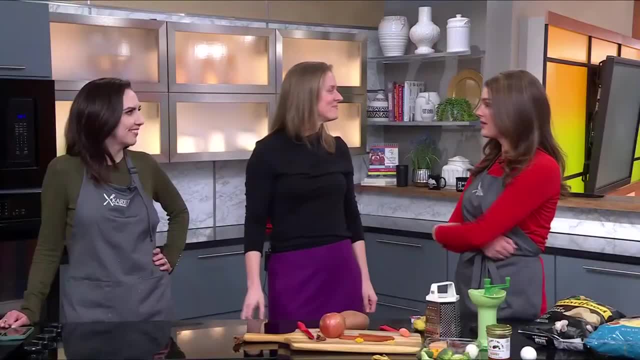 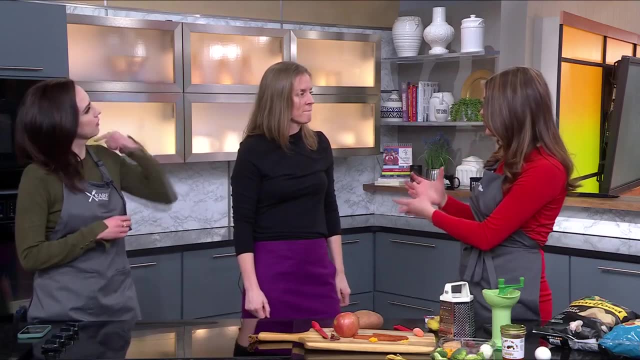 yeah, so that's the four four-year-old or higher. yeah, sorry, sorry guys. well, you're both eight gadget. i'm curious too, because you're busy: you're working in the er specifically with pediatric, so young kids, what is something you wish you could tell parents who come in and they're like: 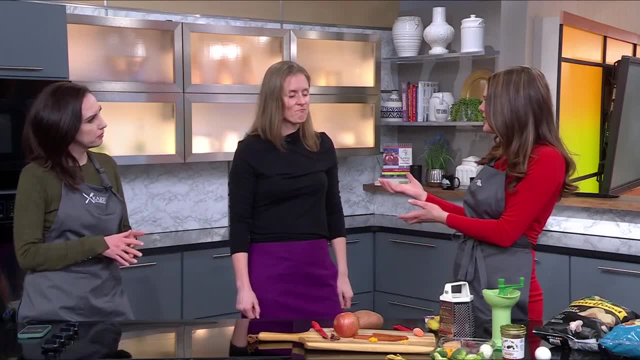 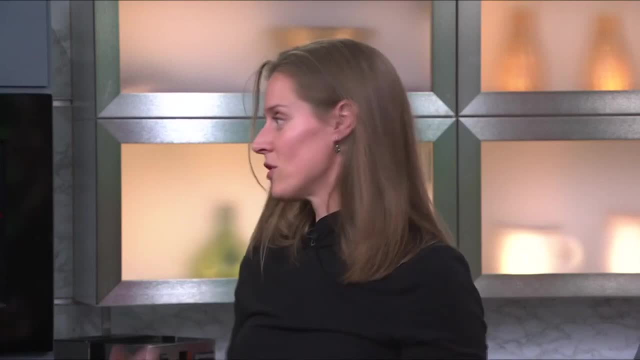 oh my god, i feel so stupid. should i have come in? should i not come in? what are you guys seeing? a lot of, yeah, i think, the main things. i would say. number one: it's never stupid to come in if you're worried. we are always there 24 7 365. that's what we're there for: to provide kind of. 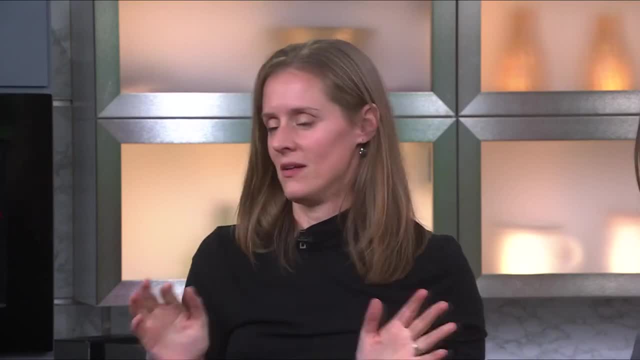 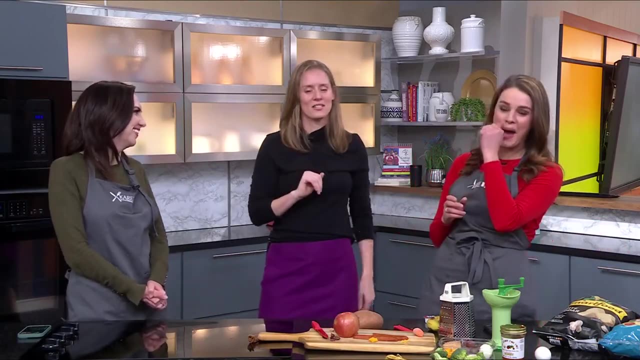 that, that guidance, that relief, that that checkup that you need when you're a parent too. so you understand the irrational fears. i'm never, ever going to roll my eyes and be like you shouldn't have come, never. so if you are worried you're not going to be able to come in, you're not going to be.